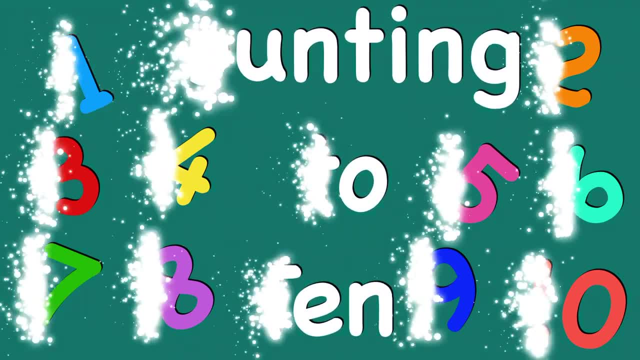 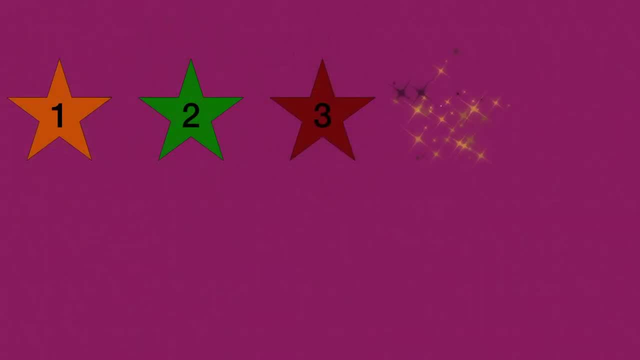 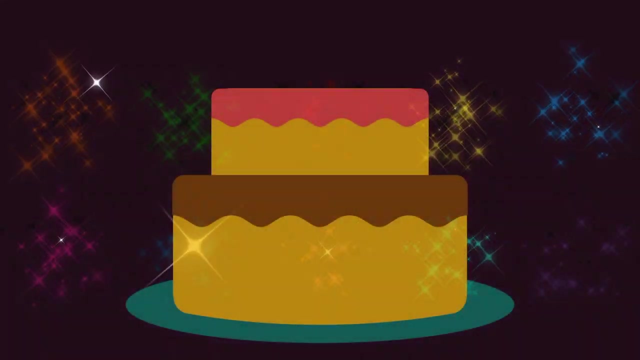 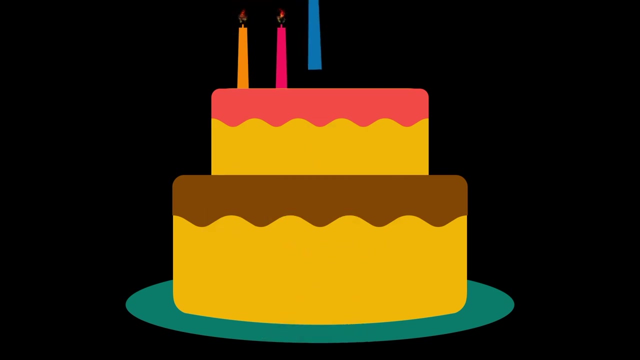 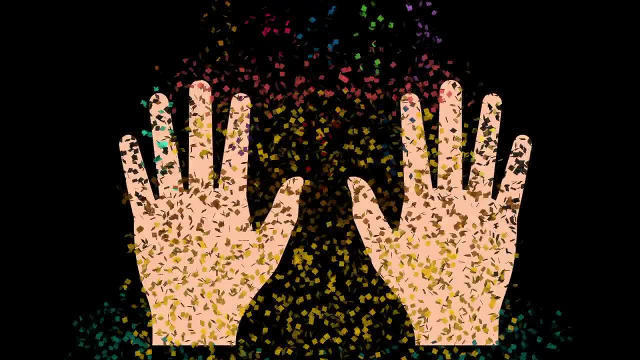 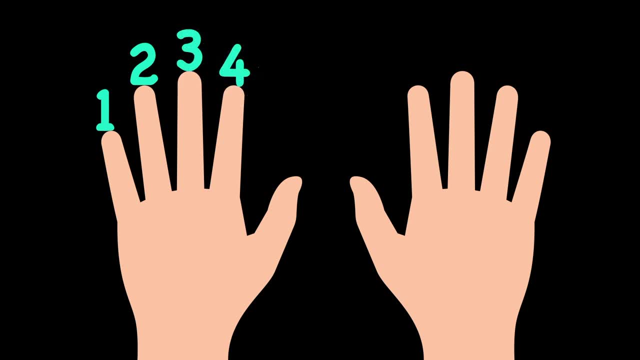 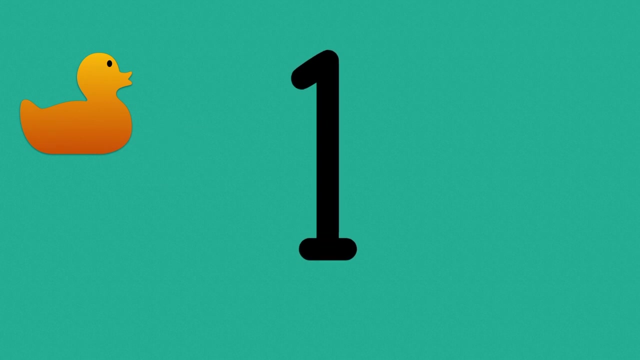 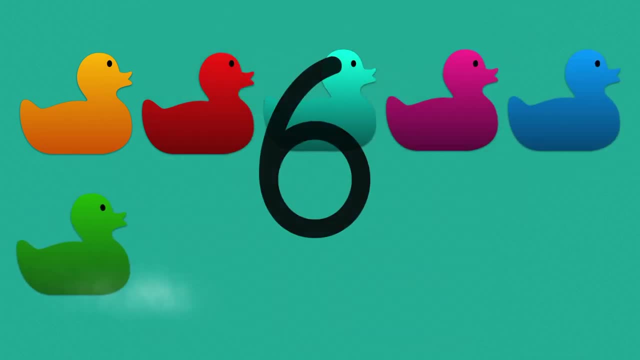 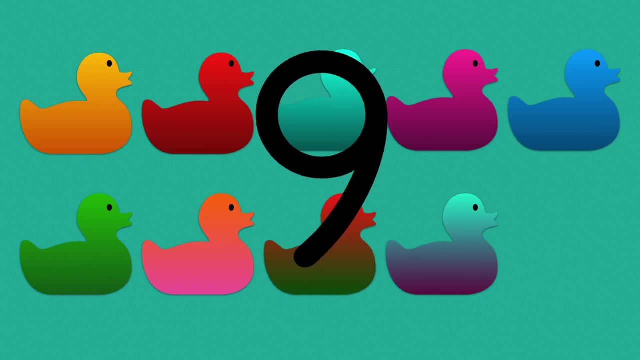 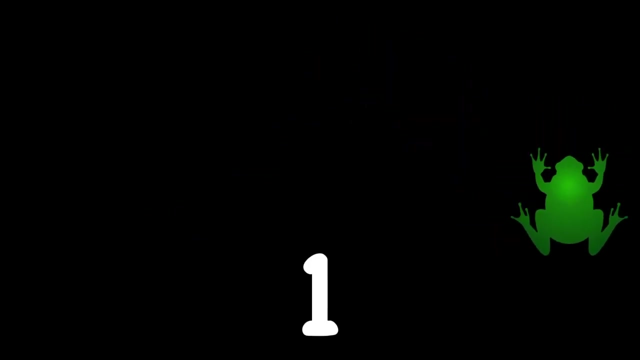 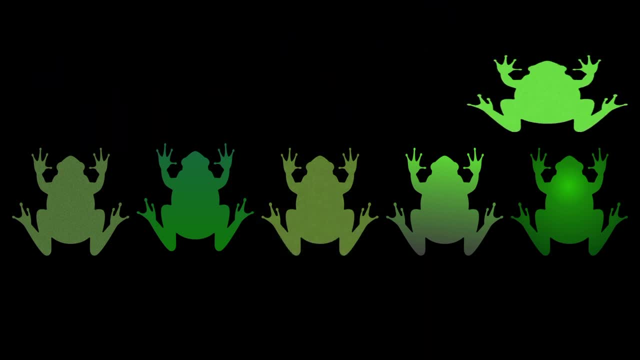 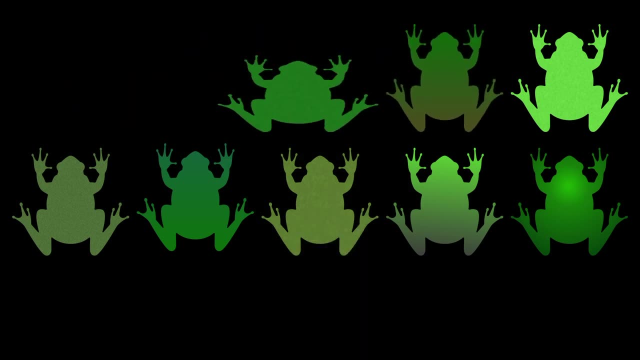 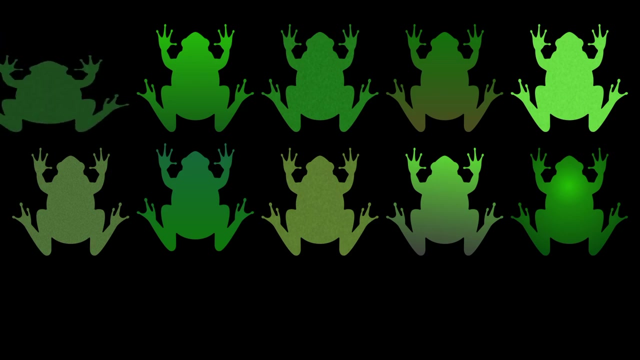 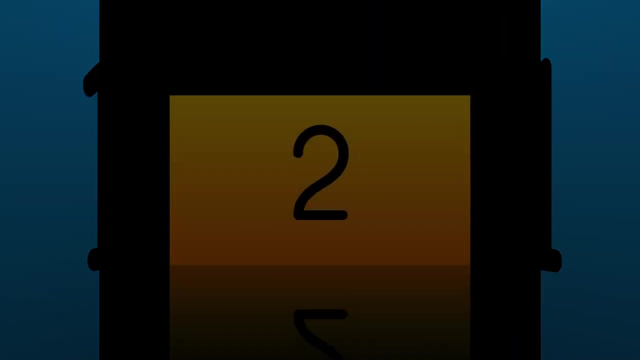 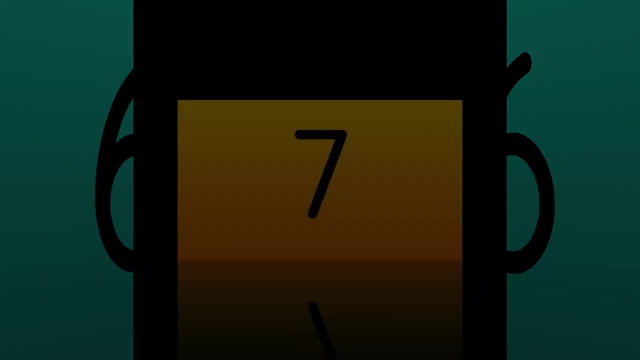 5,, 6,, 7,, 8,, 9, 10..